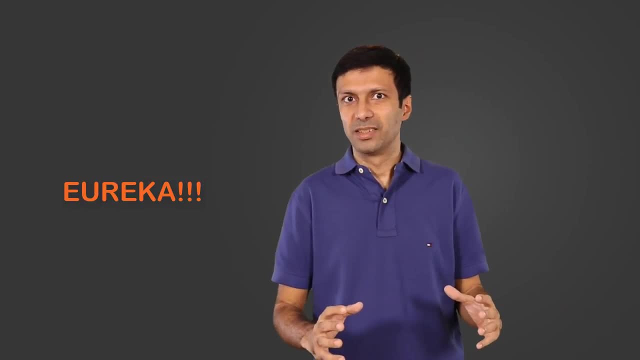 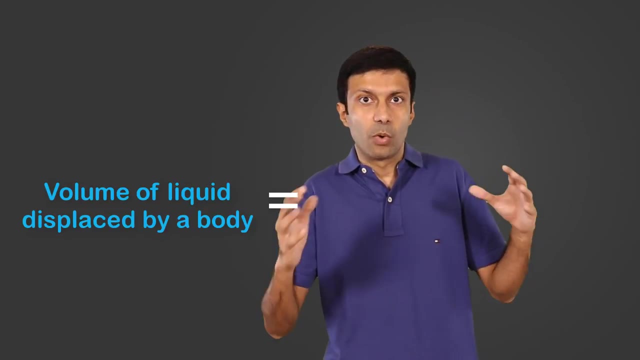 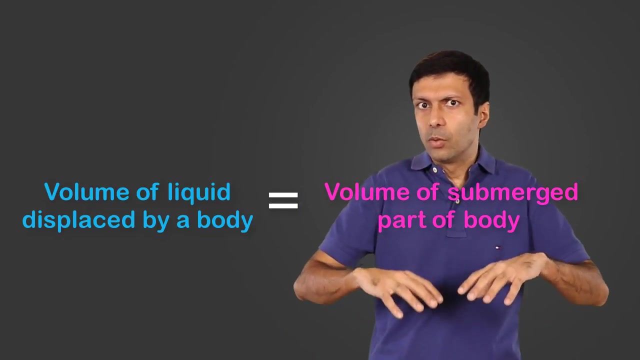 And then he had this Eureka moment. He discovered that the volume of the liquid displaced by a body is equal to the volume of the submerged part of the body. So if the entire body is under water, then the volume of the liquid displaced will be the volume of the body. 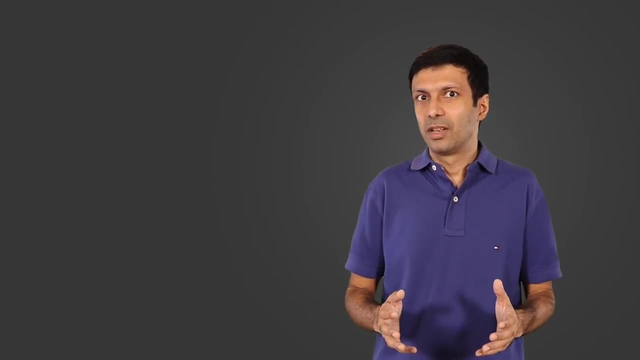 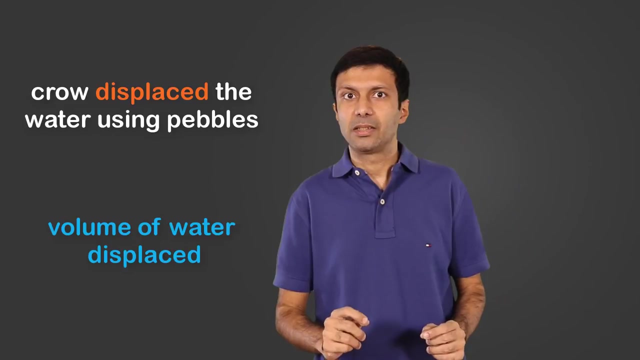 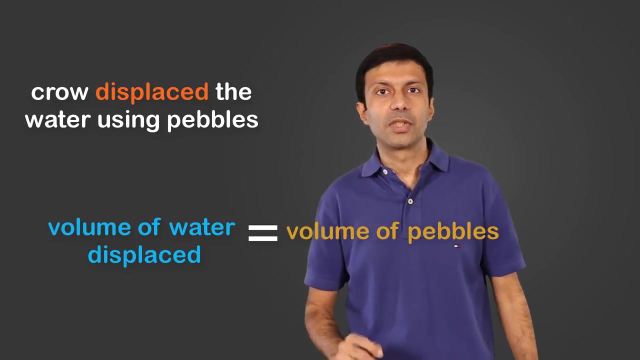 And the crow used this concept in the crow and jug story to push or displace the water up. So then the volume of the water displaced was equal to the volume of the pebbles. Let's understand this concept with the help of some experiments. 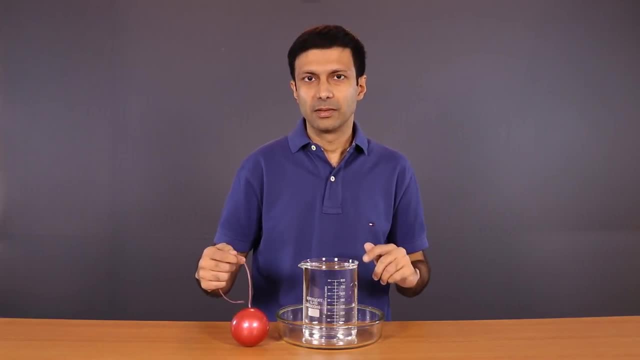 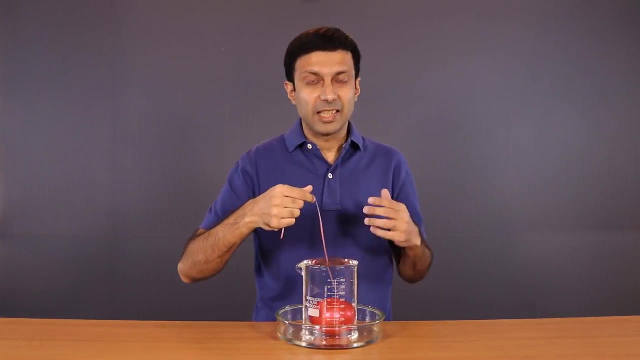 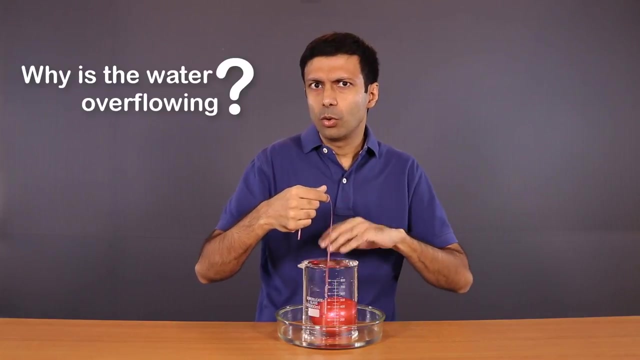 I'm going to lower this ball into this beaker full of water like this And, as expected, you saw that the water overflows into the bowl here. Now why is that? Why is the water overflowing? It's because the ball is squeezing the water. 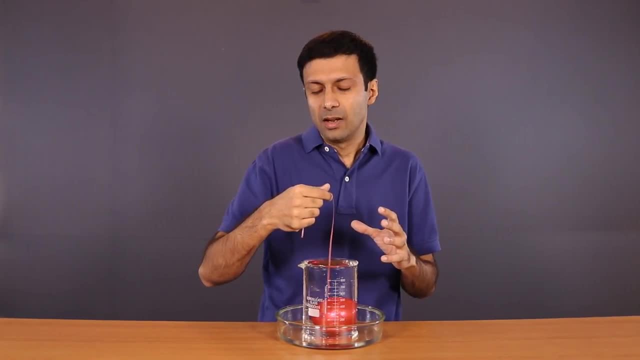 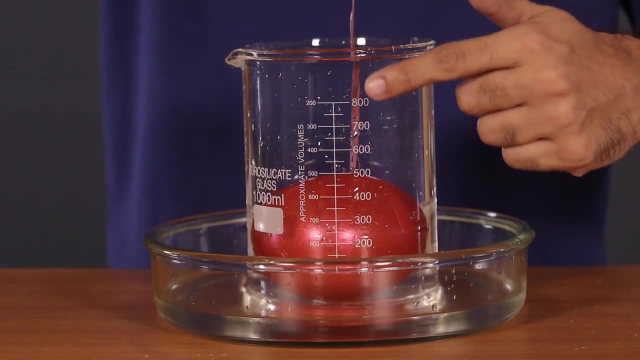 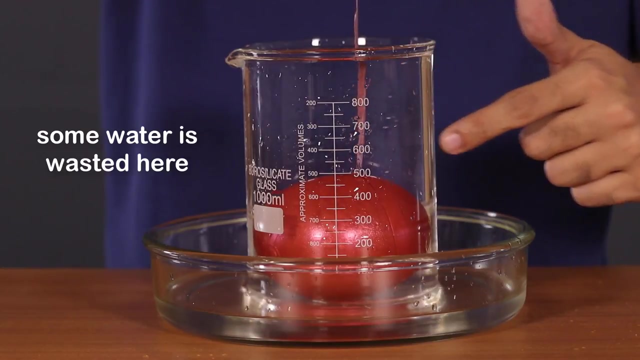 out. There's no more space, right? But it's hard to measure the volume of the water displaced accurately Because, as you can see, all the water has not gone into the bowl here. Some of it is still sticking to the beaker, So some water is wasted here. So let's try this. 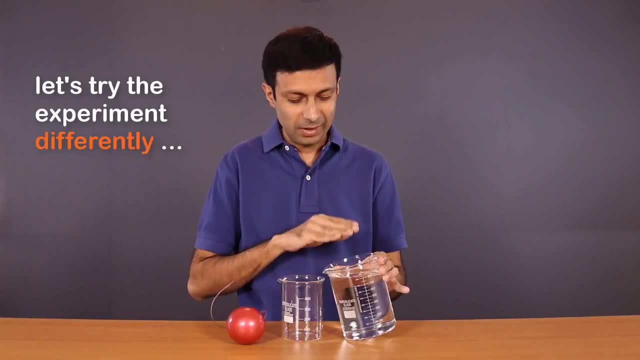 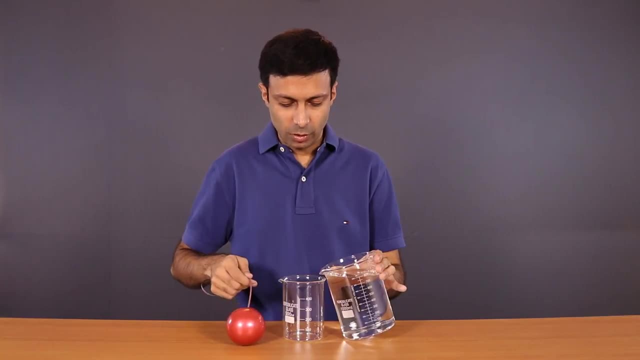 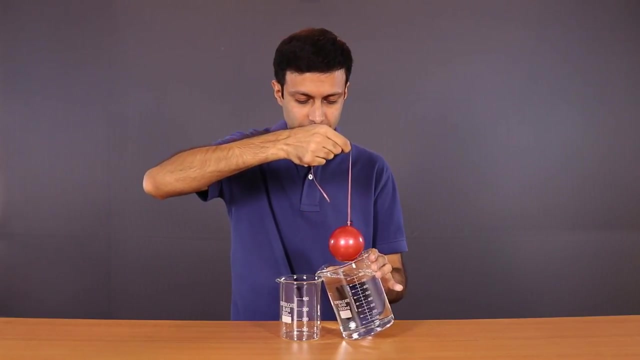 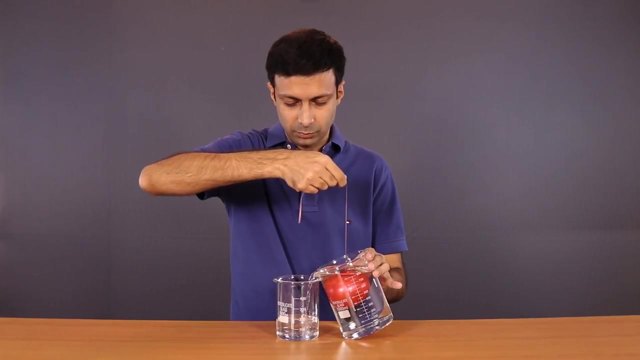 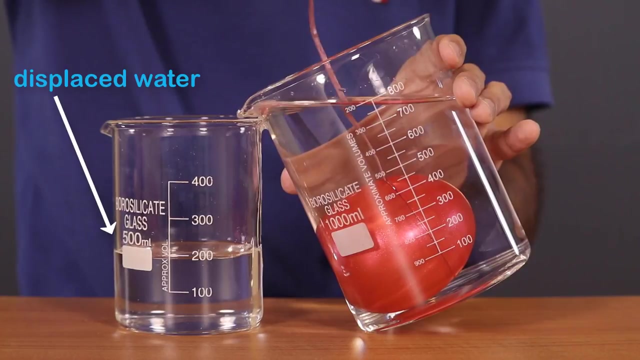 experiment differently. So now I'm going to tilt this beaker so that the water overflows into the smaller beaker here, So let's go ahead and do it one more time. So I'm going to lower the bowl again. So, as you can see, this bowl has displaced water into the smaller beaker. 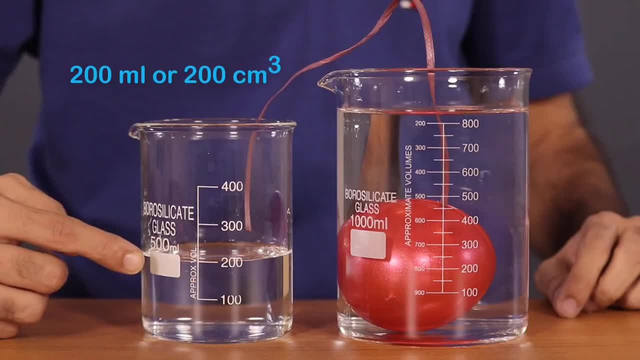 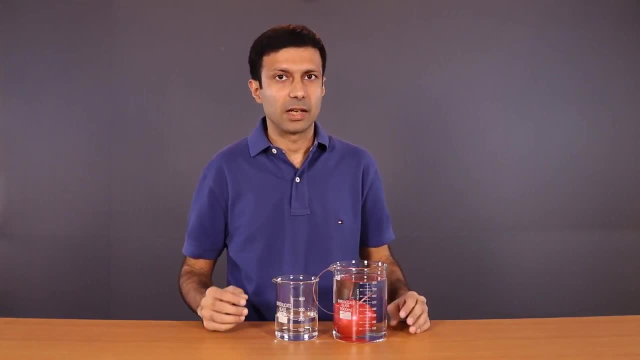 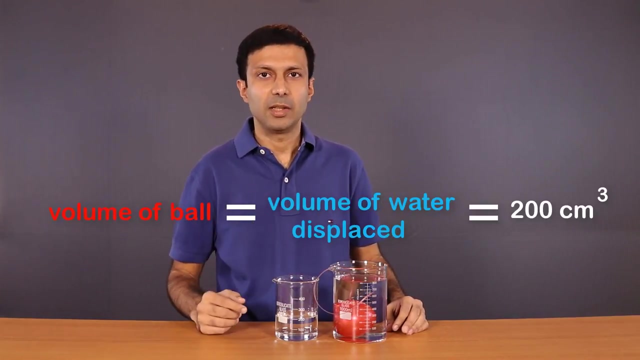 Now, what is the volume of the water displaced? It's 200 ml or 200 cm3 of water. So, by Archimedes' first discovery, the volume of this bowl is the volume of the water displaced, which is 200 cm3.. 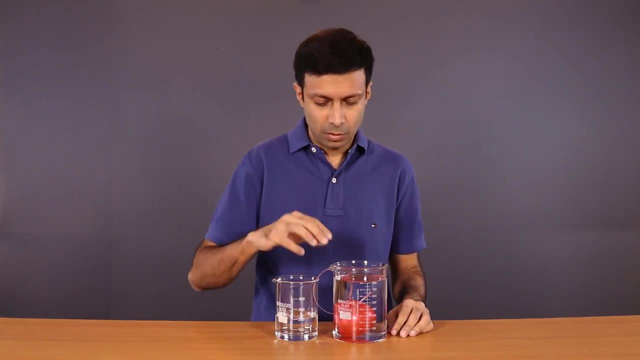 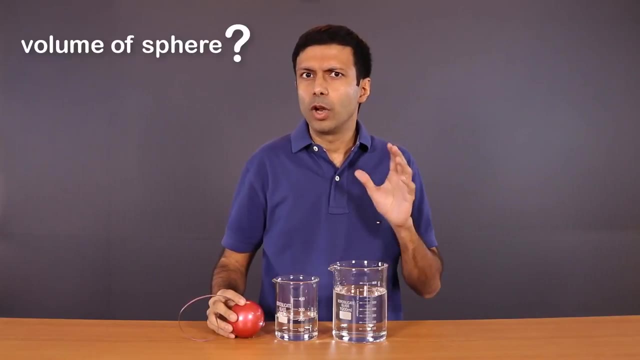 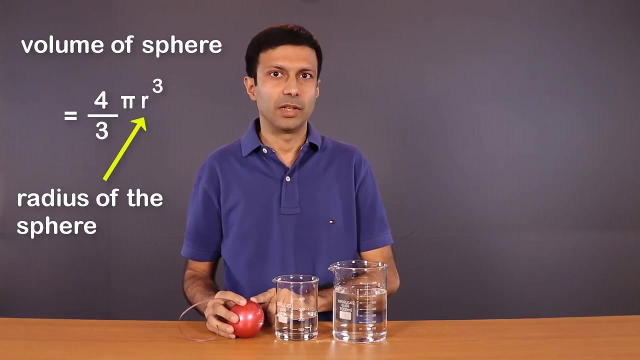 Now how can we verify that? So we know that this bowl is a sphere. Now what is the formula for volume of a sphere? It's 4 by 3 pi r cube, where r is the radius of this sphere. So I've actually gone ahead and checked that. 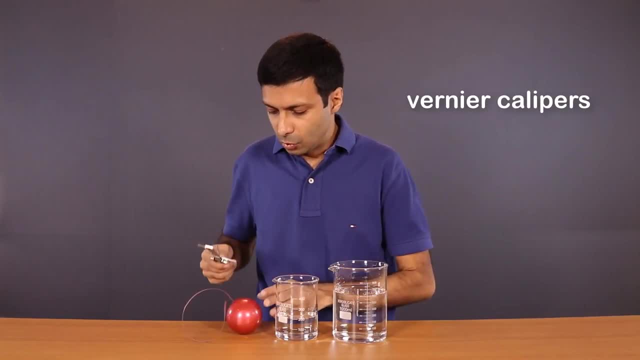 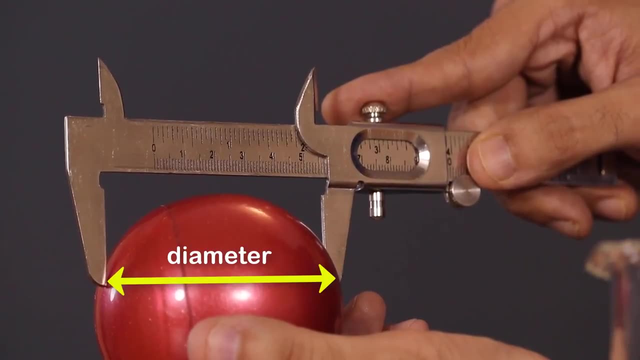 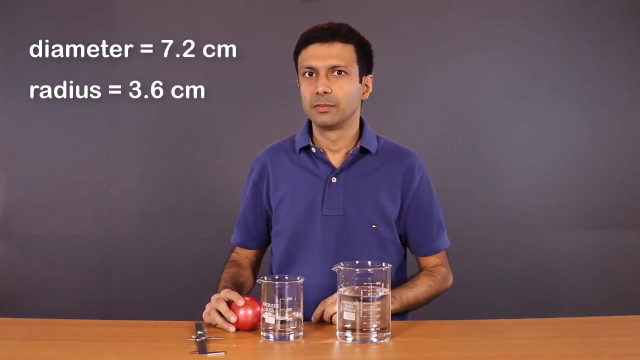 with the help of a virtual machine. So I went ahead and measured the diameter of this bowl here like this: And the diameter of the bowl is 7.2 cm, So the radius is 3.6 cm. And now, if I use the formula 4, by 3 pi r cube. 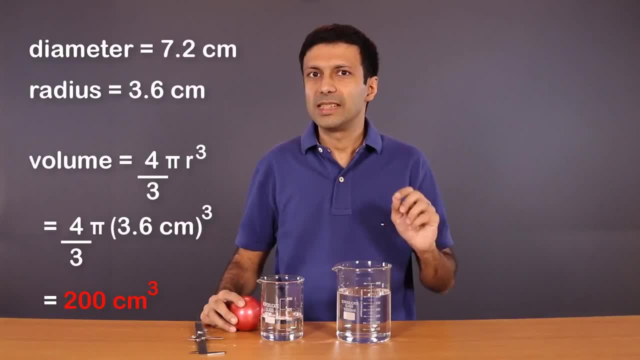 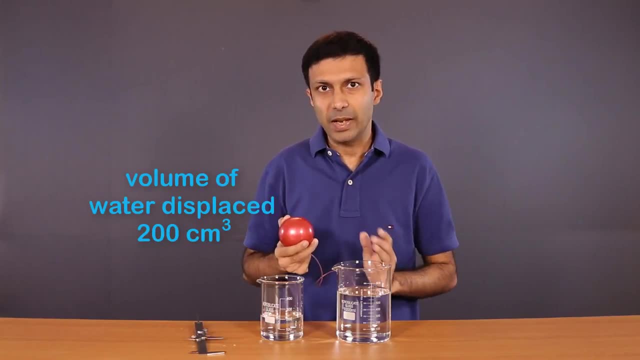 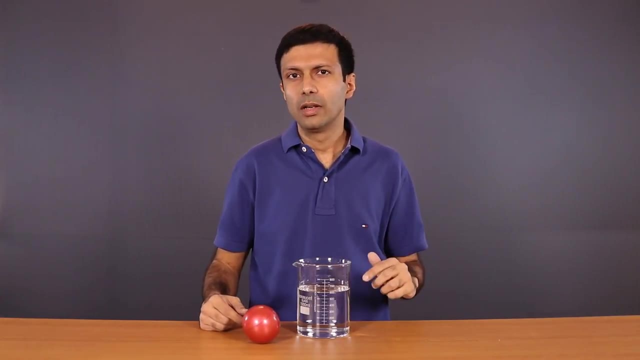 I'm getting the exact same volume: 200 cm3.. So Archimedes' discovery is correct, that the volume of the water displaced by this bowl is the volume of the bowl itself. We can actually find the volume of the bowl in an easier way. 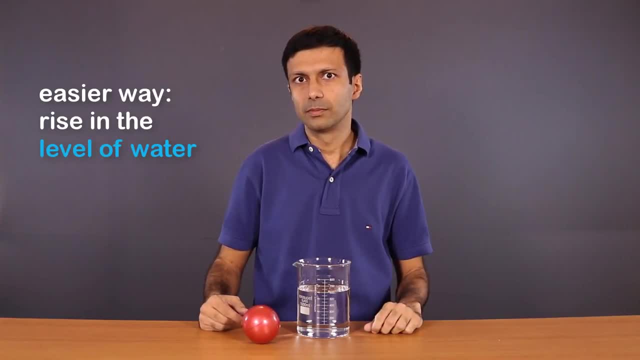 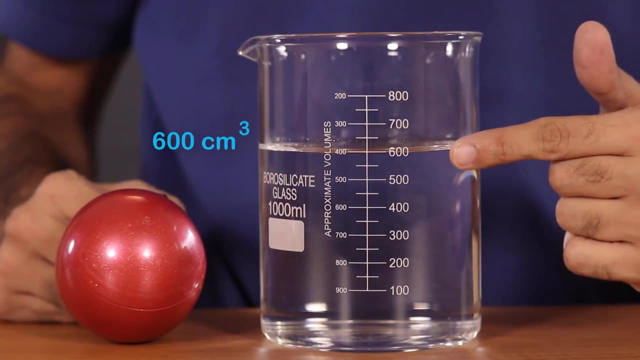 by measuring the rise in the level of the water. So, as you can see, the initial volume of the water here is 600 cm3.. So I'm going to lower this bowl one more time and keep an eye on the level of water. 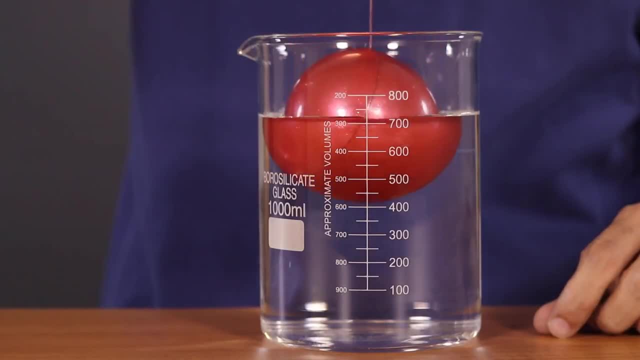 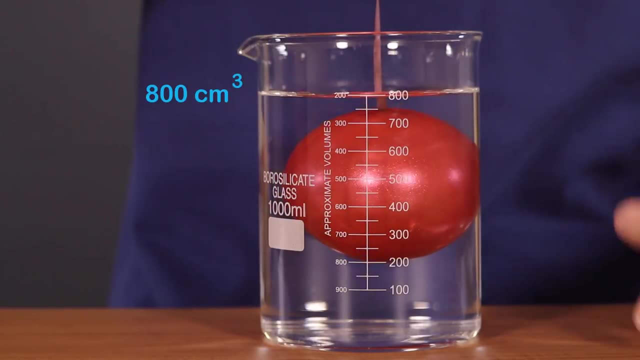 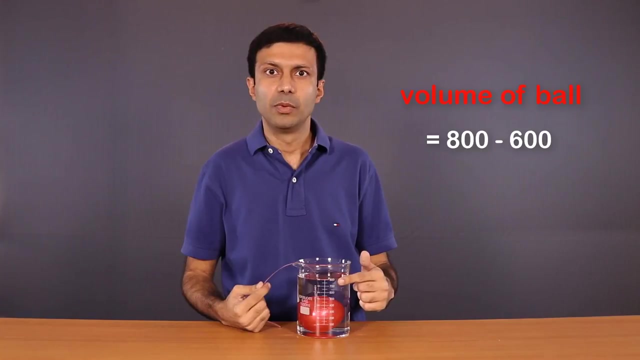 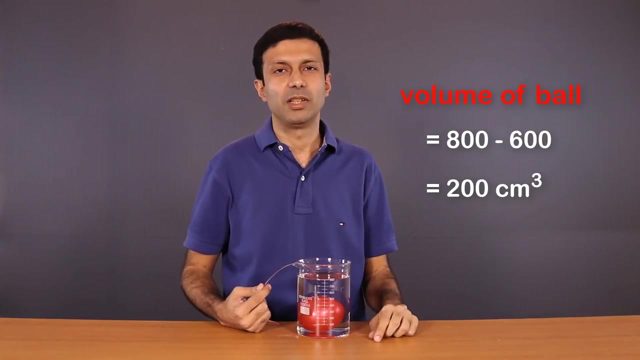 So, as you can see, the level of water has risen to 800 cm3.. So the difference in the volume of water is the volume of this bowl, So which is 800 cm3 minus 600 cm3.. So the volume of this bowl is again the same thing: 200 cm3. 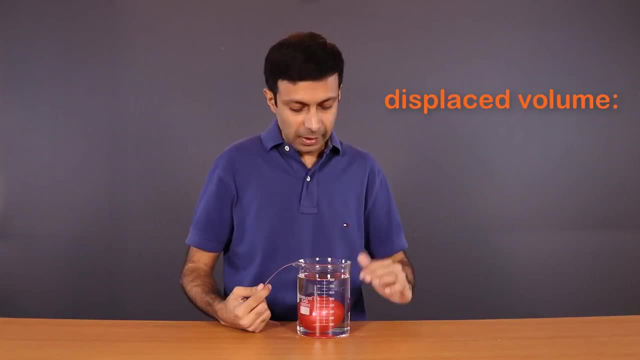 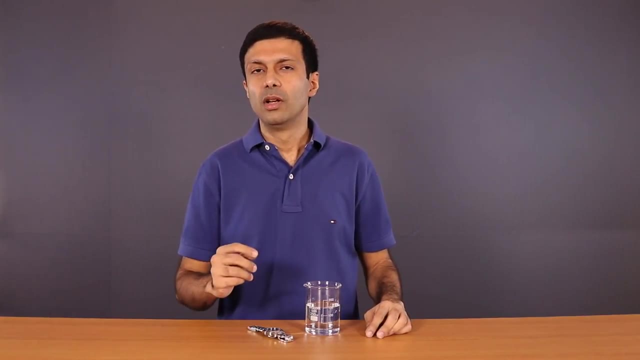 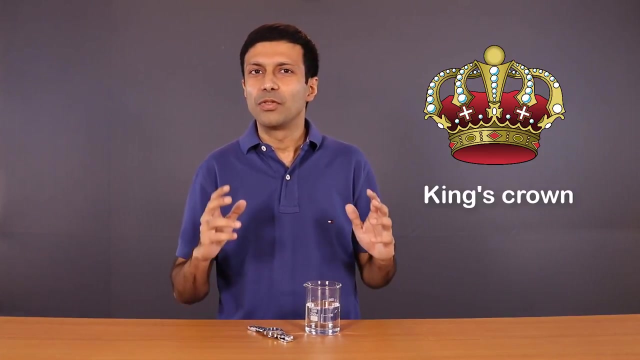 So displaced volume is basically the volume that rises or the volume that overflows. This discovery is very useful for measuring the volume of irregular solids. Archimedes used it to measure the volume of the king's crown. Now I don't have a crown, so I'm going to use my watch instead. 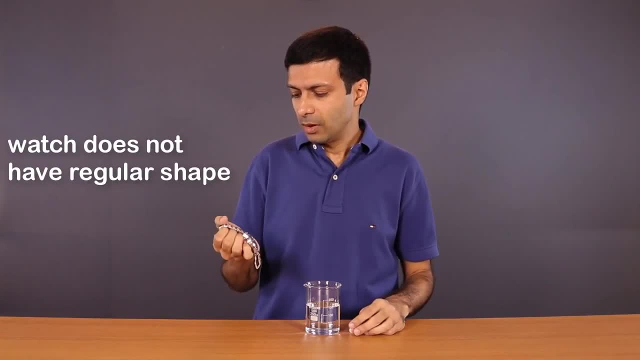 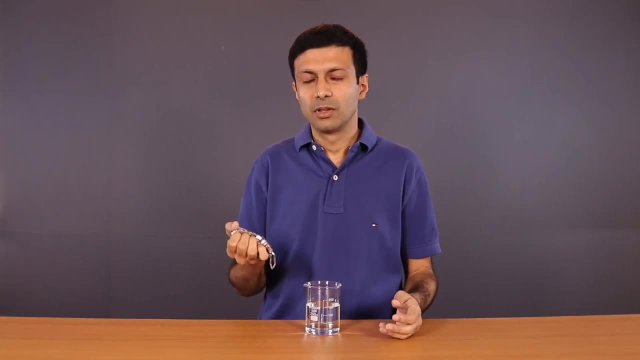 So my watch doesn't have a regular shape. I can't use the formula of a cuboid like L, x, B x, H, or that of a sphere. So what am I going to do? I'm going to lower it into this beaker of water. 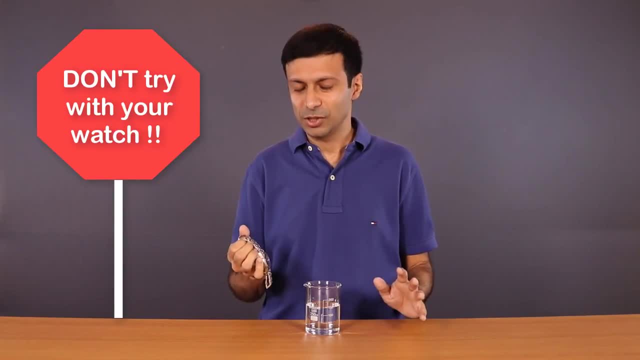 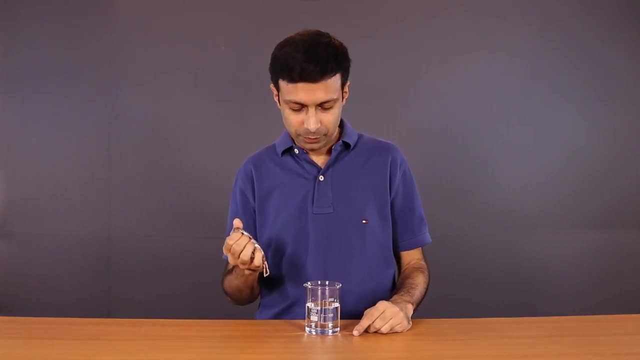 Now I don't want you to try it because I don't want you to spoil your watch. So let's go ahead and try Now. what is the initial volume of water here? As you can see, it's 150 cm3.. And I'll lower my watch into that. 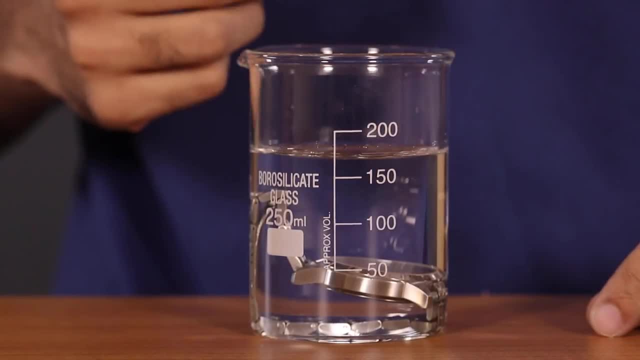 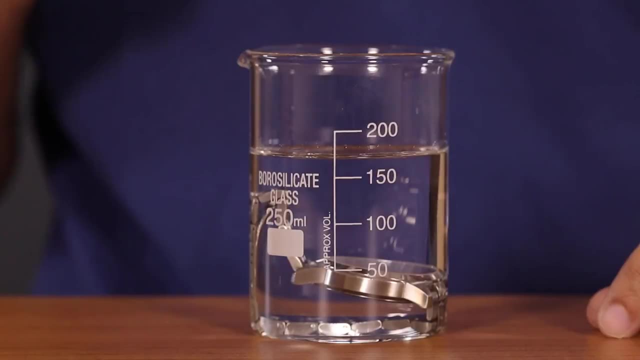 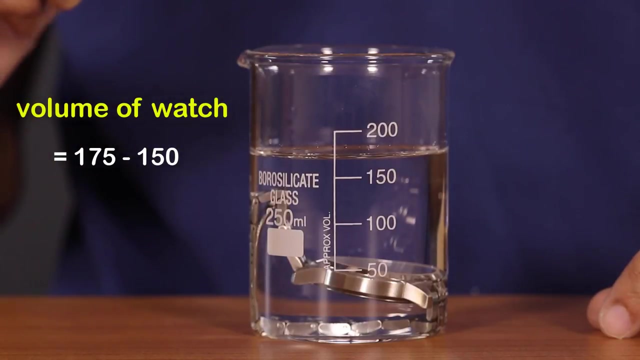 And I'll lower my watch into this beaker So, as you can see, the water level has gone up to 175 cm3.. So what is the volume of my watch? It's the difference in volume, That is, 175 minus 150, which is 25 cm3.. 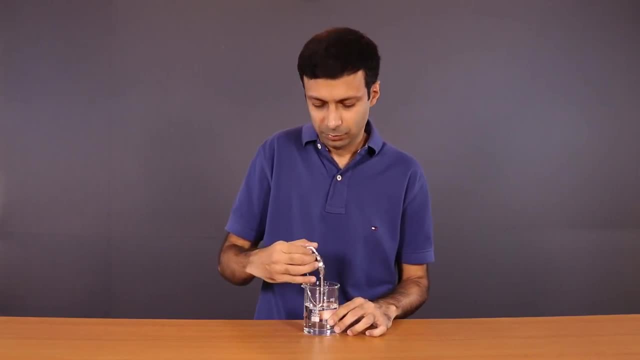 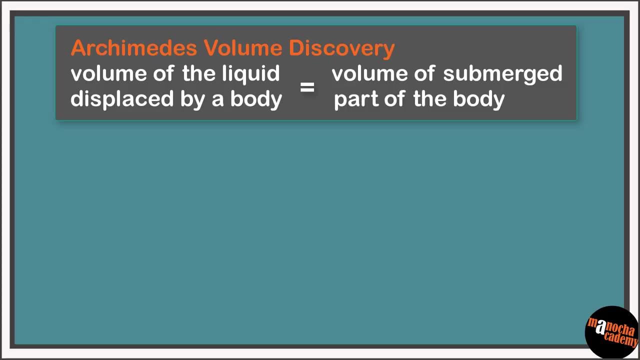 So my watch has a volume of 25 cm3.. I hope it's still working. So let's place Archimedes' volume discovery on our concept board. When a body is completely immersed in the liquid, we can say that the volume of the liquid displaced is the volume of the body. 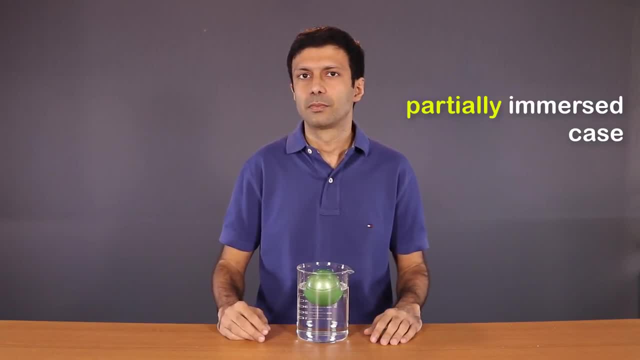 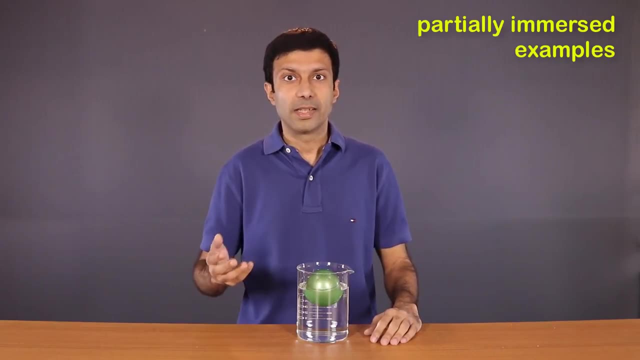 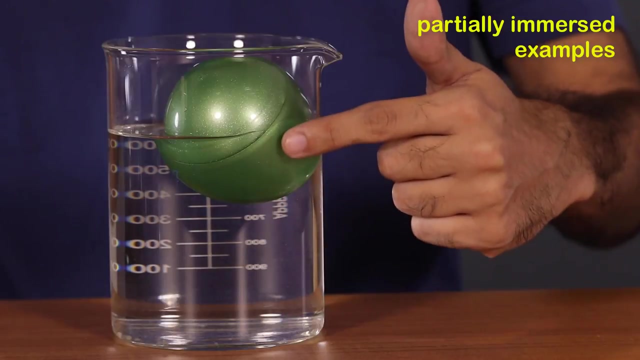 Now let's check the partially immersed case. So what are some examples of objects that are partially immersed in water? One example is a floating ball like this- As you can see, it's partially immersed in water. Or an iceberg is another example of an object partially immersed in water. 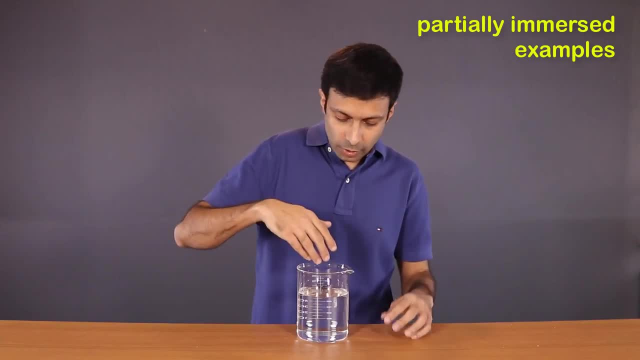 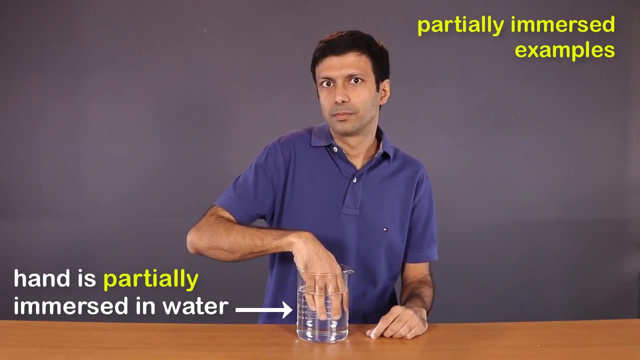 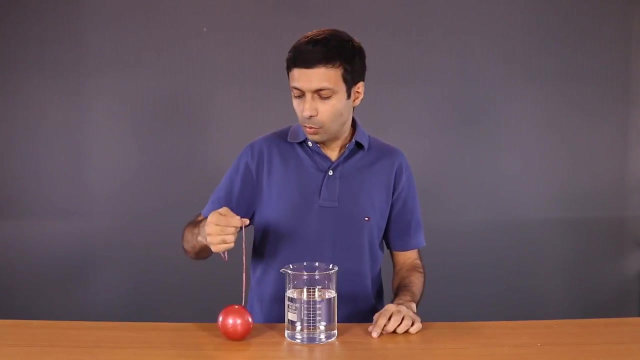 Now, if I take out this ball and if you put your hand in the water like this, so you can see that your hand will be partially immersed in water. So let's understand the partially immersed case. with the help of an experiment, With the help of this string, I'm going to partially immerse this ball into the beaker of water here. 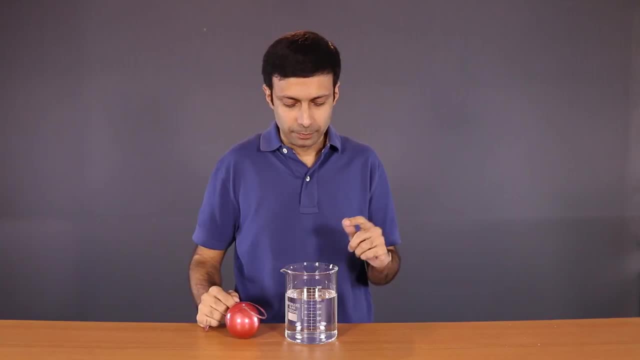 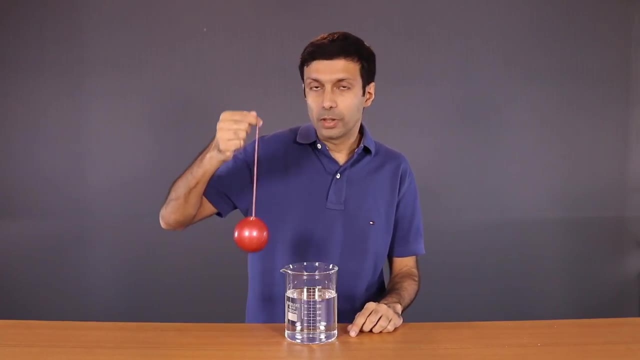 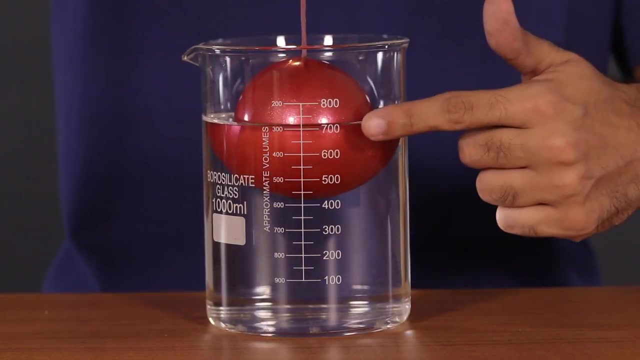 But first let's check what is the initial volume of water. As you can see, it's 600 cm3.. Now I'm going to lower the ball so that it's partly immersed in water. So what is the volume of water now? 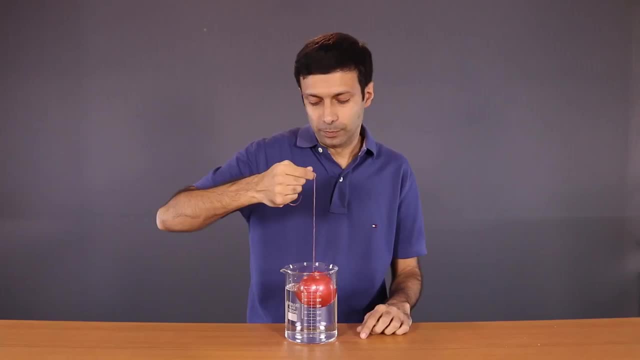 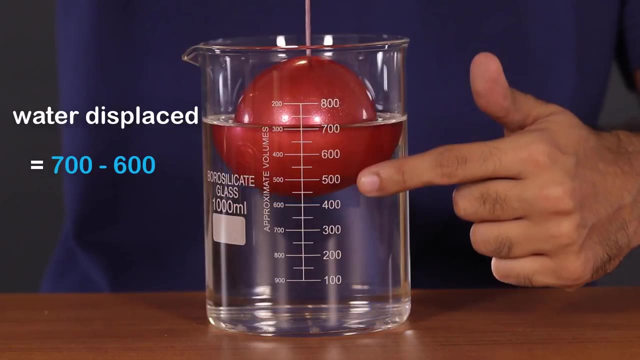 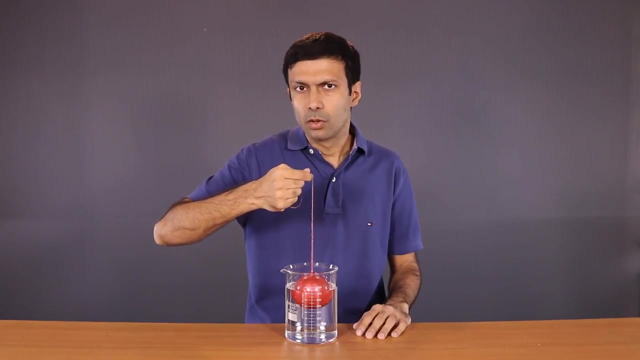 As you can see, it's 700 cm3.. So how much water has been displaced? So it's 700 minus 600 cm3. So that's 100 cm3 of water has been displaced. So what is the volume of the ball which is under the water?